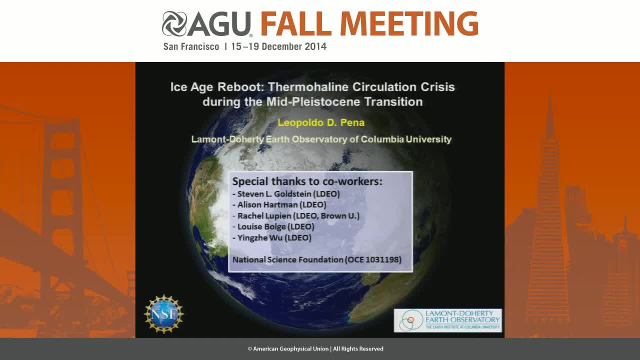 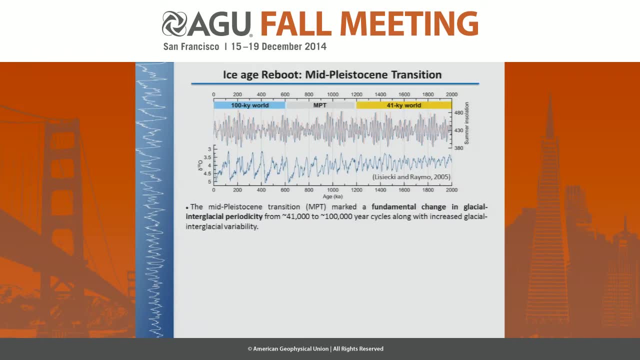 but also the people like Allison Hartman, Rachel Lupin, Luis Bolcha and Inge Obu, all from Le Mans. So the mid-Pleistocene transition is mostly marked by a fundamental change in the glacial-interglacial periodicity. 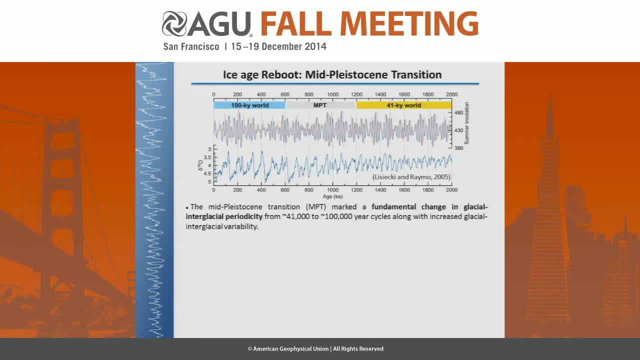 which shifts from 41,000 years to 100,000-year cycles, and it's also accompanied by increased glacial-interglacial variability. This is clearly seen in a wave-lutenspectral analysis on this benthic isotope stack over the last two million years. 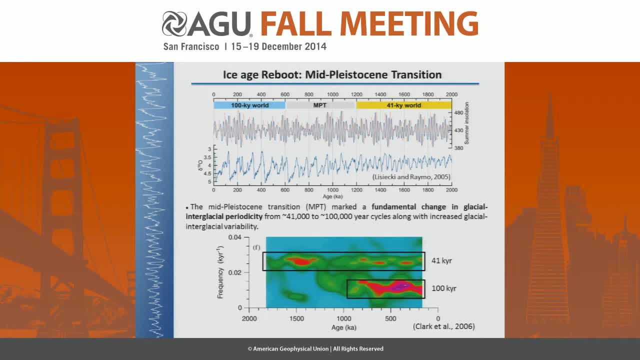 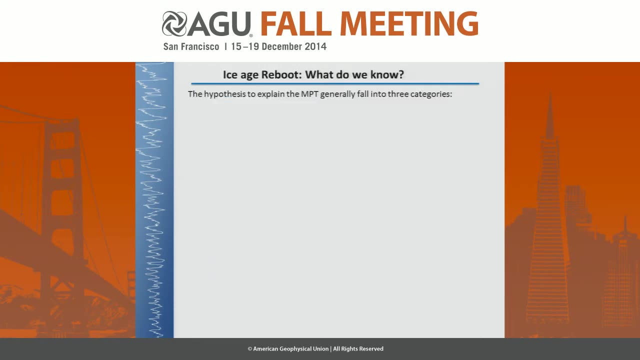 where you can clearly identify these 41-kiloyear frequency down here before one million years, and then sometime around this interval, the 100-kiloyear periodicity shows up. So there's been many hypotheses to explain why this happened and it would be completely impossible for me to go in detail into all these hypotheses in this talk. 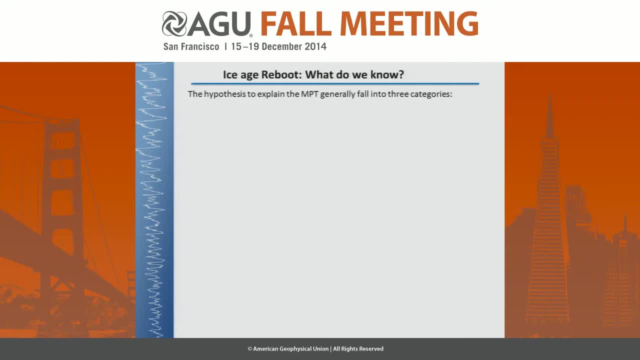 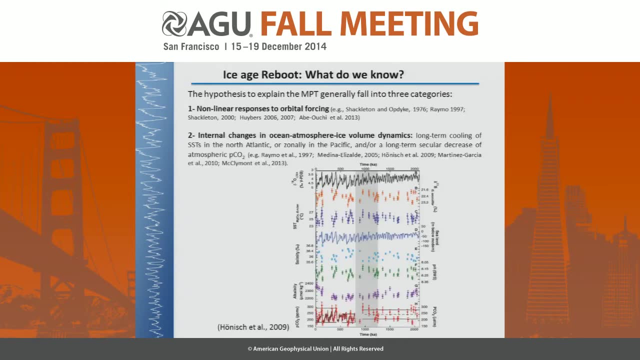 But in general, all these potential explanations fall into three different categories, namely nonlinear responses. So the first one is: what are the changes in the glacial-interglacial dynamics in the ocean atmosphere due to orbital forcing? In second place, internal changes in the ocean atmosphere, ice volume dynamics such as, for instance, long-term coolings of SSTs in the Atlantic and the Pacific. 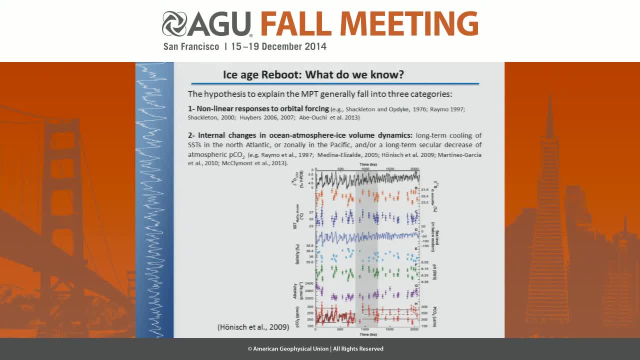 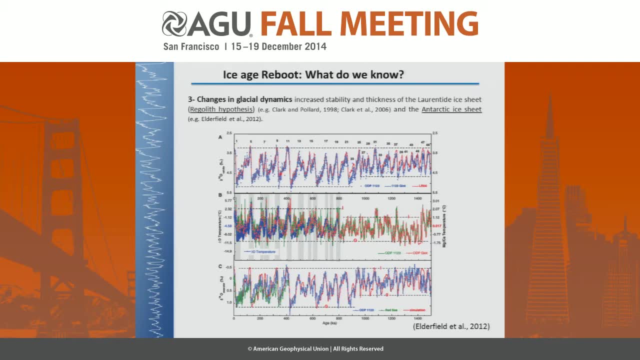 but also long-term secular changes of atmospheric CO2, like those shown in this work by Barbel Honish in 2009.. On the third group of hypotheses, we may have changes in glacial dynamics. In particular, important in this category are the increased stability and thickness of the Laurentian Sea. 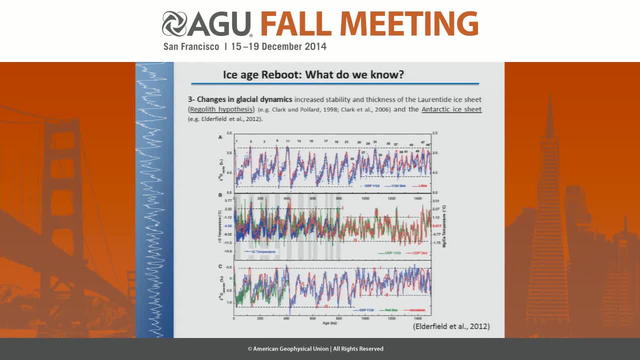 as well as the increased stability of the Antarctic ice sheets. the so-called Regolith Hypothesis, But also, more recently, work by Harry Alderfield and others, also highlighted the importance of the Antarctic ice sheet and how the stability of this big ice mass might have impacted the NPT during this time. 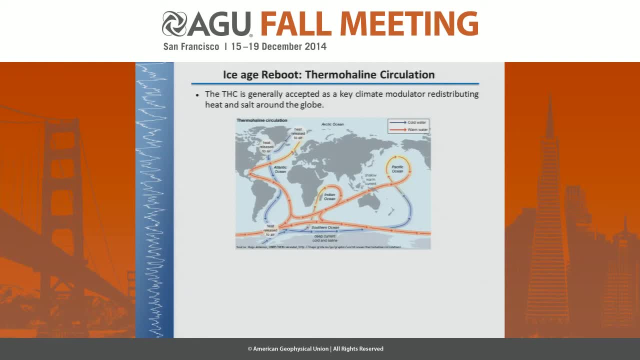 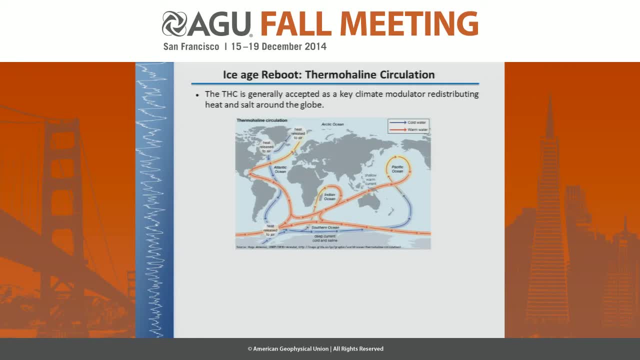 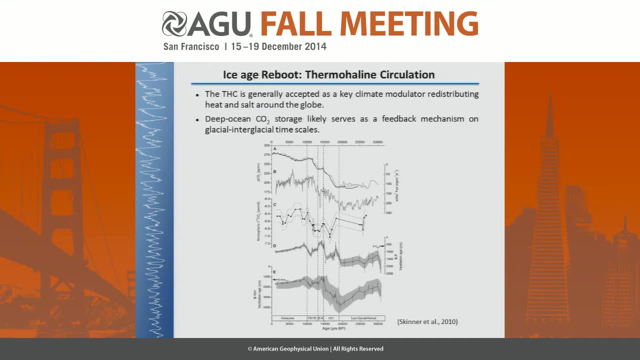 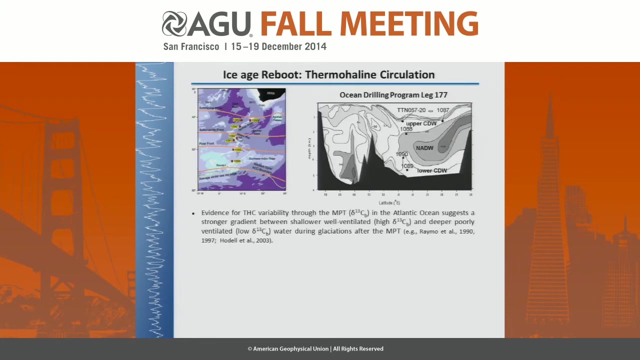 We know that nowadays these mechanisms generally accept. as a key climatologist, We have had some reserv marry of celestial, of vitamins, cm, th, p. The answer is yes, we do, and they are mostly all based on benthic carbon isotopes In particular. I'm going to be showing here some data from the Cape Basin. this set of 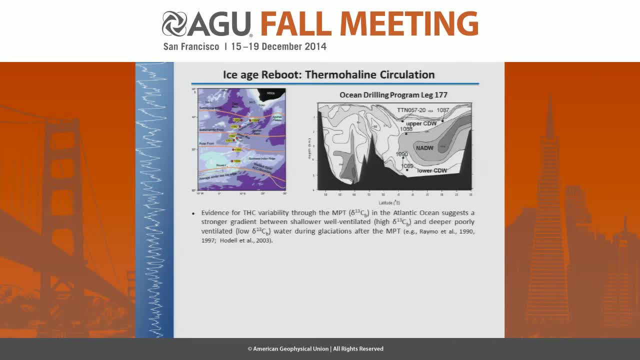 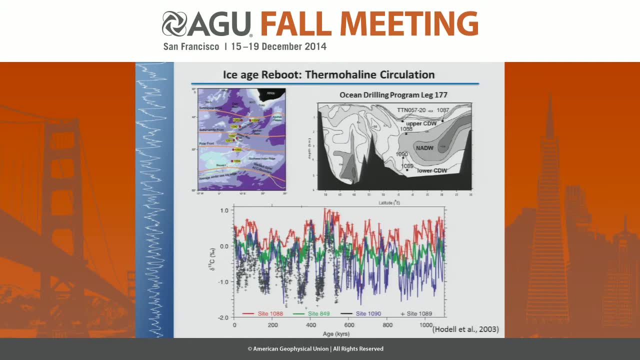 ODP cores 1088, 1090, and 1089, and the benthic carbon isotopes on these three cores essentially show an increased carbon-13 gradient between what they call a shallow, well-ventilated water versus a deeper, poorly-ventilated water. before and after the NPT. 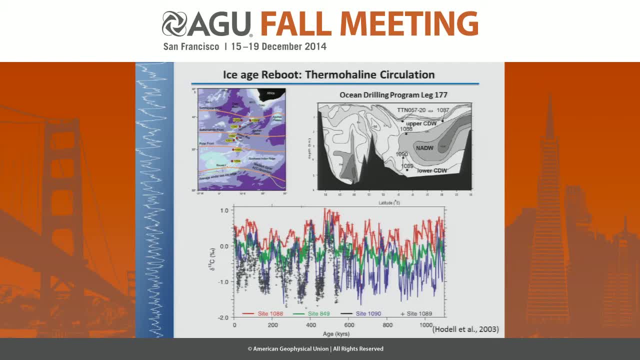 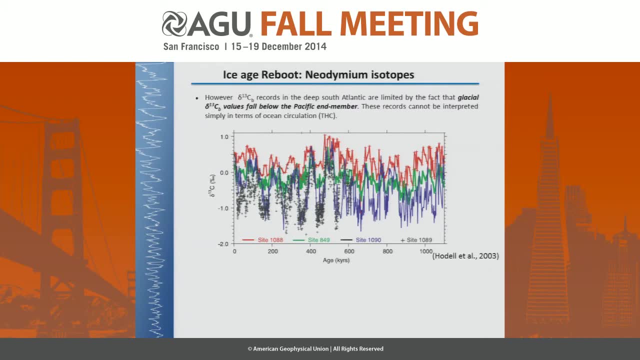 Essentially, the gradient between these two water masses increases as we go from pre-NPT periods of time into post-NPT time periods. But, however, these benthic carbon records in the deep South Atlantic are limited by one observation, and that's the fact that the glacial carbon-13 values fall below the 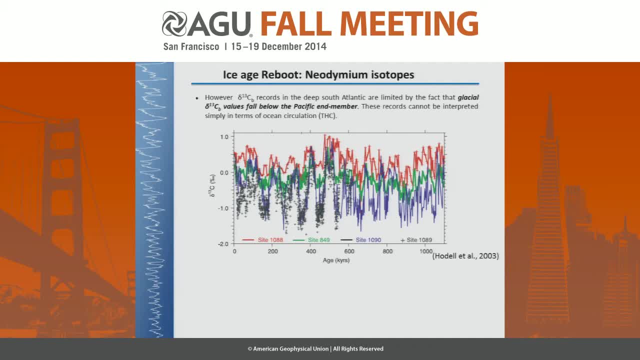 Pacific and member. If you look here- sorry- If you look at Site 849 in the Pacific, it's right in the middle. So Site 1090,, which is the deeper one of these two have all through the last million. 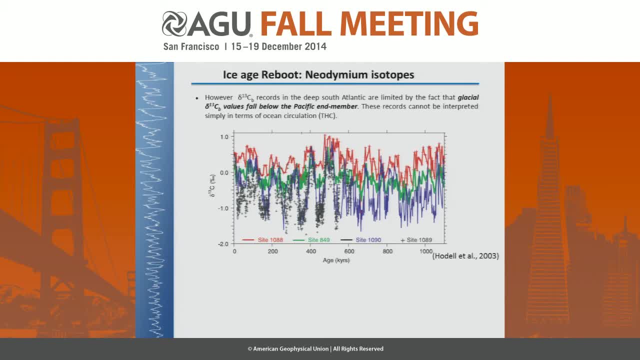 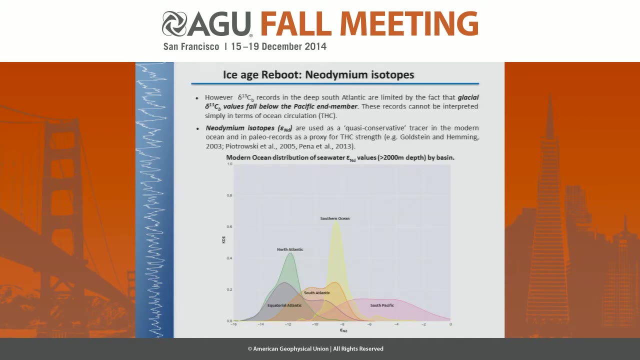 years more negative values than the Pacific and member. Therefore, it's extremely complicated to interpret this just simply in terms of strength of ocean thermohelm circulation. So what can we do about that? Well, we can use another set of tools like, for instance, neodymium isotopes, which are 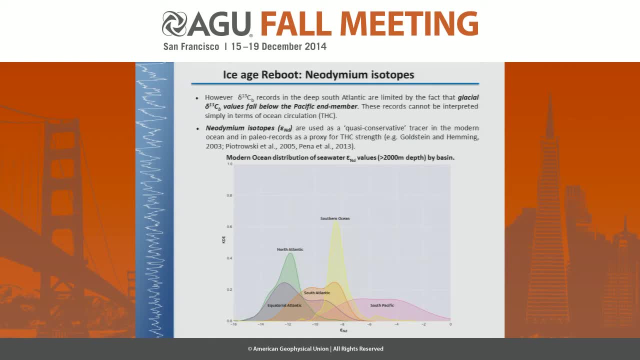 quite Quasi-conservative tracers, both in the modern ocean also used in paleo records as proxy for thermohelm circulation strength. And I'm not going to go in great detail how neodymium isotopes work, but just to give. 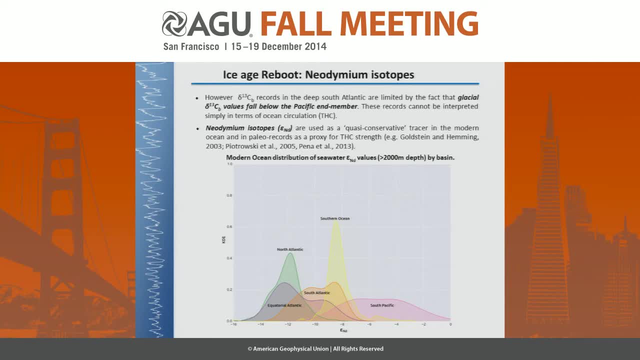 you a brief overview. if we take all the modern ocean seawater epsilon-diemion values below 2,000 meters and we plot the distribution by basin, we see that the North Atlantic is characterized by fairly negative epsilon-diemion values and as we move south, the equatorial 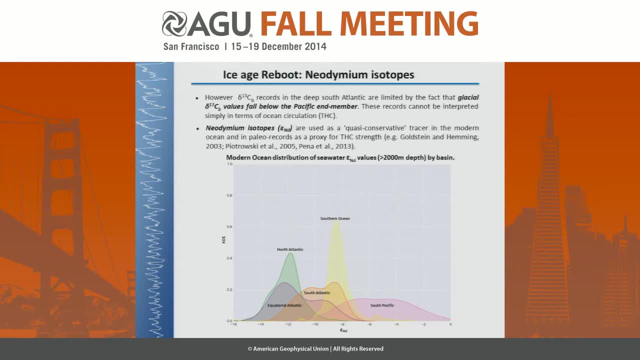 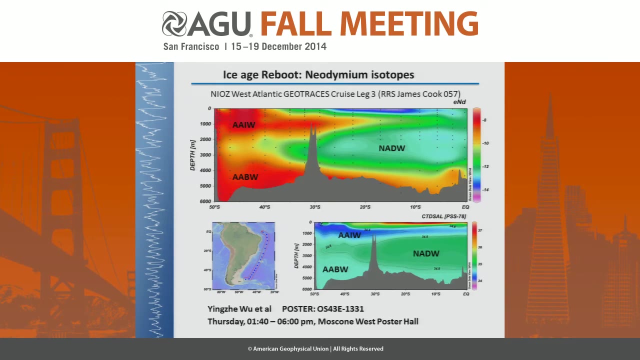 Atlantic, the South Atlantic And the Southern Ocean. the values become progressively more positive until we go into the South Pacific. Just to give you a much clearer view of how this actually works in the ocean, I'm showing this geotracer section along the South Pacific. 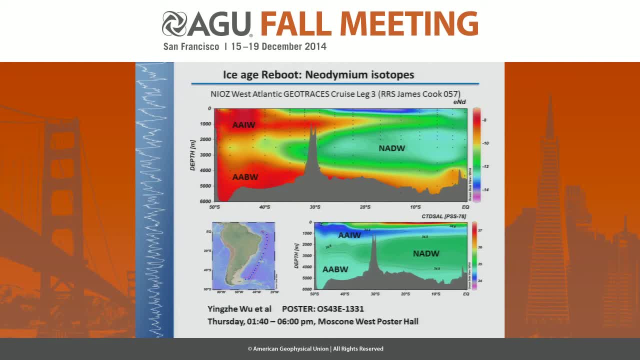 This is an amazing work done by Injo Buen. She'll be presenting a poster later this week on Thursday afternoon, so I really encourage you to stop by and check it out. But what we see here There is epsilon-diemion at the top, salinity at the bottom and we have this negative tongue. 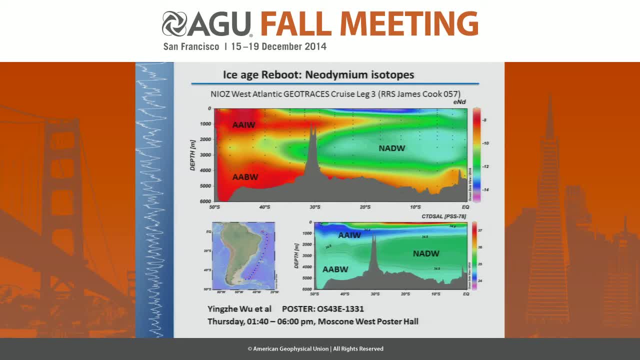 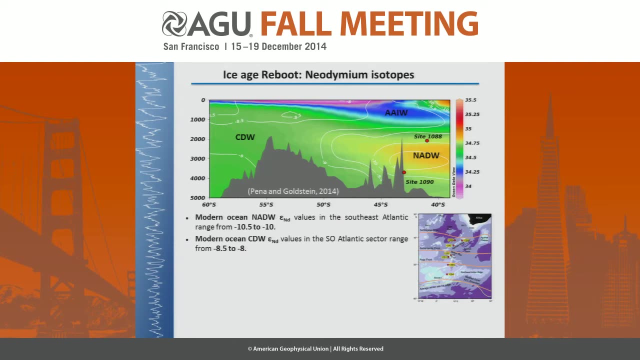 of NADW moving south here values around minus 12 or so, Antarctic Indonesian water and Antarctic bottom water moving north with more radiogenic values. So, going back to these Cape Basin sites, we just decided to concentrate on site 1088 on. 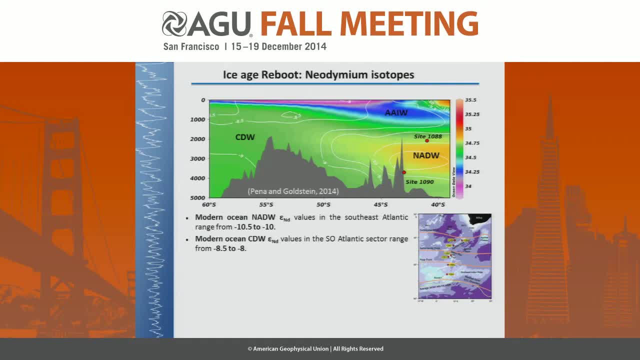 top of the modern NADW core in the South Pacific, In the southwest- sorry, in the southeast Atlantic and the deeper site 1090 down here And the modern ocean. epsilon-diemion values in this region range from minus 10, minus. 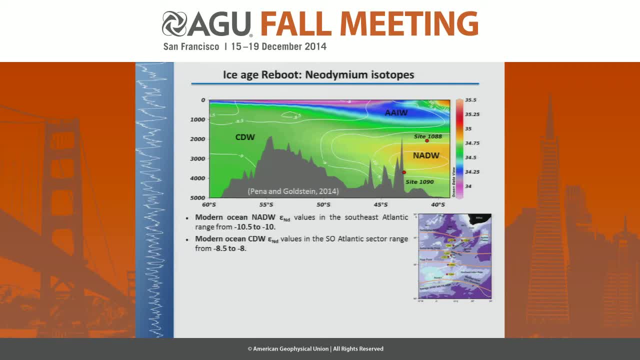 10.5 for the NADW and minus 8 to minus 8.5 in the Southern Ocean waters in the circumpolar deep water. So essentially, if we were to look into the pillar records in these two sites, we would. 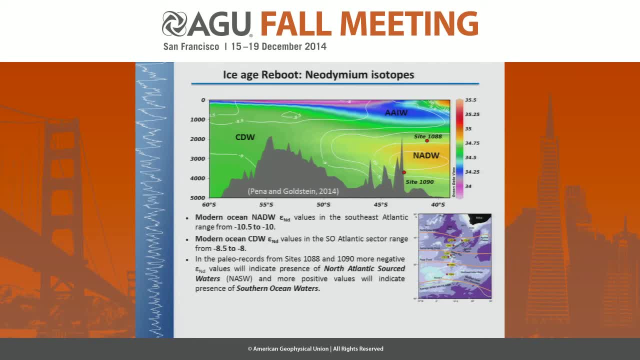 interpret more negative epsilon-diemion values to indicate more northward North Atlantic source water is getting into the south Atlantic, whereas more positive values will indicate the opposite: more presence of southern ocean waters. here. And for those of you interested in more details on this work, I'll encourage you to check. 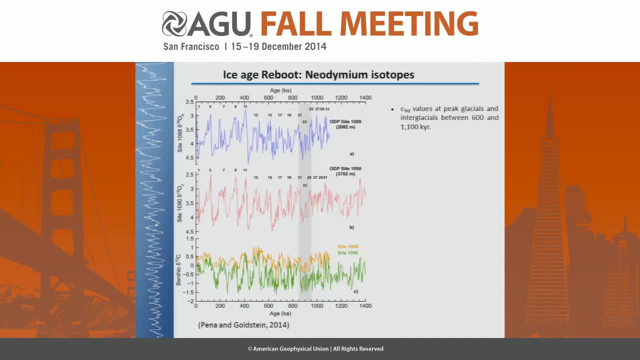 on this paper that we published earlier this year. So let's get into the data Here. time scale: 1.5 million years, roughly Ben thick oxygen isotopes for site 1088 and site 1090.. Remember intermediate depth: 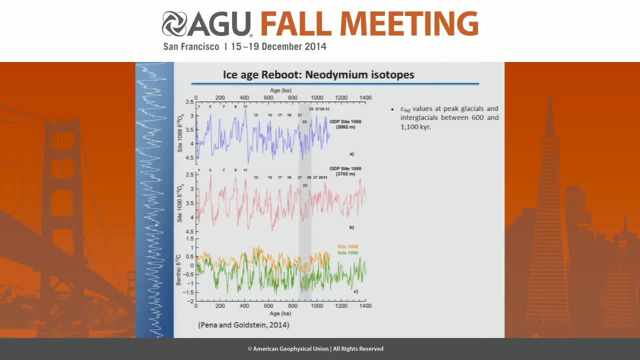 2,100 meters meters and deeper side, 3,700 meters. so what we decided to do here was: let's just concentrate on the peak glacial and peak interglacial intervals at these two sites from the time until between 600,000 and 1.1 thousand kilo years. so 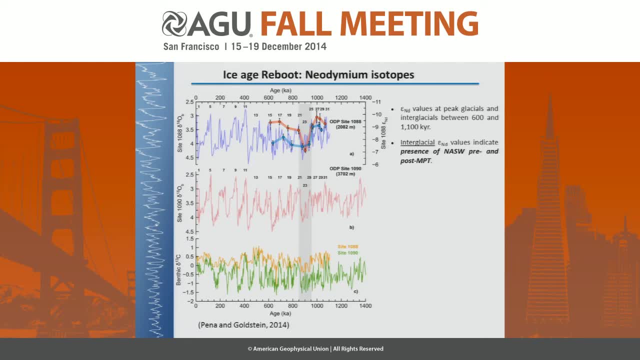 these are the results. in red you see epsilon-edimin values on this axis here for the interglacials down here, and the blue dots correspond to the glacial periods. so what's interesting when you first look at this data is that let's just look first at interglacial data. all the interglacial data seem to fall on. 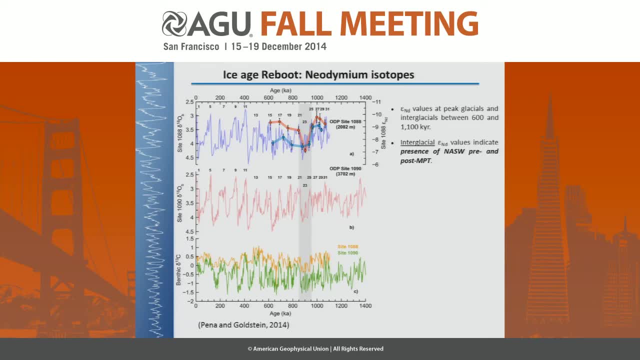 the same range between minus 10, minus 9.5 here, with the only exception of this data point. that corresponds to MIS 23 here. but when we look at the at the glacial data, the value is, you know, before, what we would call the pre-MPT time period, the glacial values. 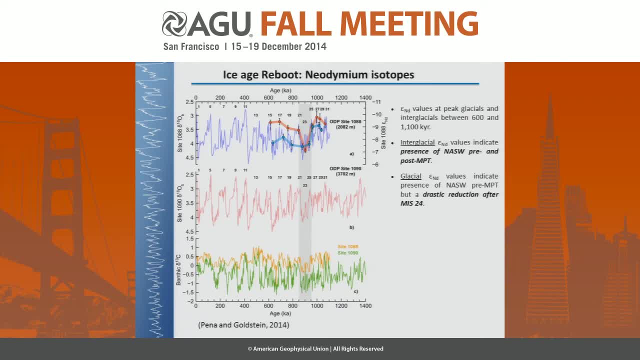 are also relatively quite negative. you know they also indicate presence of North Atlantic source waters during this time interval. but there is a drastic reduction in the epsilon-edimin value here after MIS 24, and then the glacial values stay at the same relatively positive level between minus. 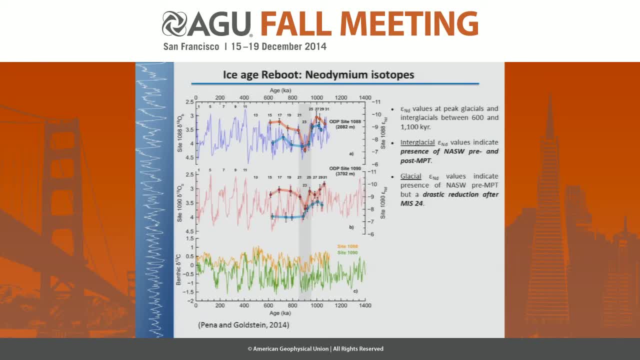 7.5 and minus N 8 and this bar and it's also shown in the deeper core with a slightly more progressive change compared to the shallower side. so what happens at interglacial, at the marine isotope stage 23, around 900,000 kilo years? well, 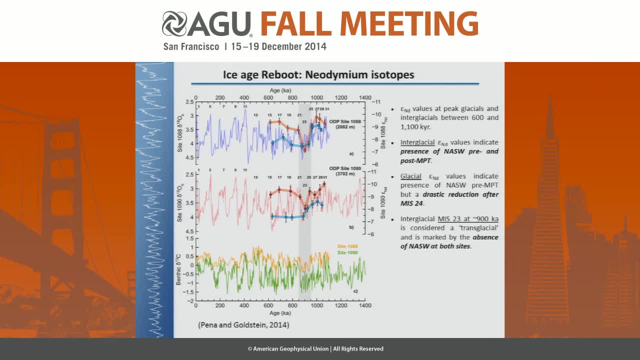 this is what is Steve Boston likes to call a transglacial. essentially it's an interglacial. that never happened and it's marked by the total absence of of North Atlantic sea North Atlantic source water at both sides. When you look at the absolute epsilon edemium values here at site 1098 and site 1090, the values correspond. 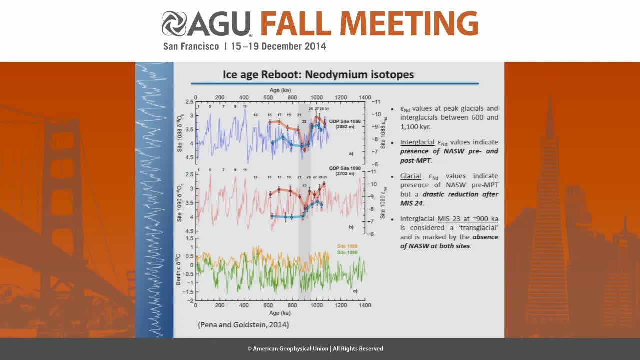 to glacial values or even more positive here, and almost the same is going on here. So we could say that, based on the- at least just based on the epsilon edemium results, the deep ocean circulation in the South Atlantic shifted from a pre-NPT very active glacial. 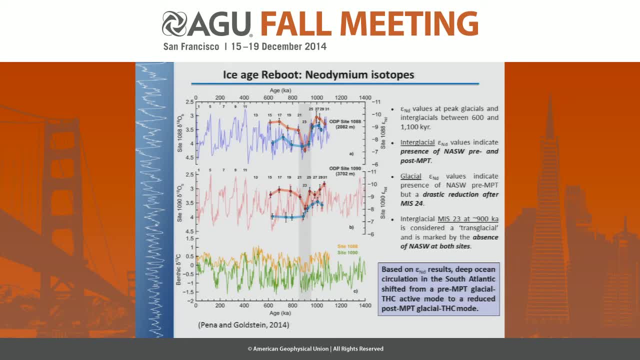 thermohaline circulation to a post-NPT reduced thermohaline circulation during glacial periods, whereas interglacials stay constant through time, with the only exception of this time, of this event at MIS-23.. So, for those of you that like to visualize it in a more cartoony way, again the time 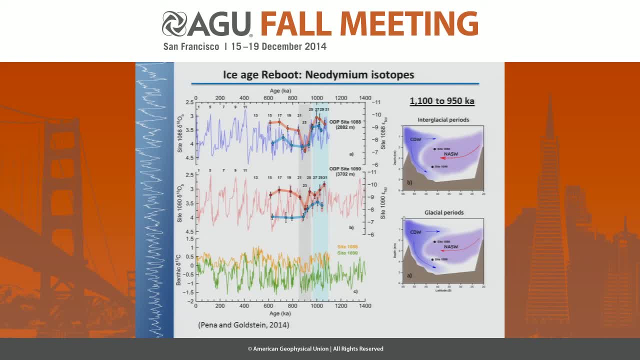 period is very important, The time period between 1.1 to 950 kilo years. We have interglacial here in red epsilon edemium values. so presence of North Atlantic source waters at both sides both during interglacial periods but also during glacial periods. 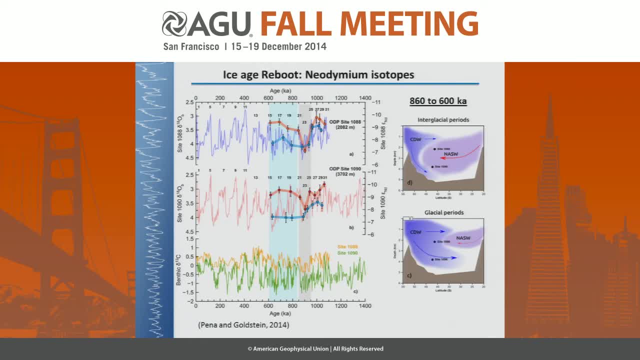 On the other side, in the post-NPT time interval between 860 and 600 kilo years, interglacials essentially stay the same, but the glacial periods are the ones that show a striking presence, and that's a much more reduced presence, of North Atlantic source waters. 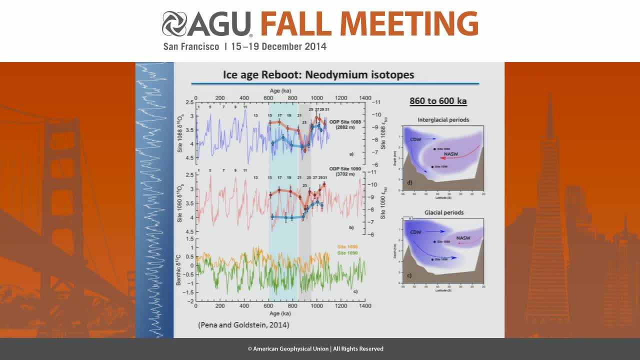 But can we quantify that? You know this is just based on epsilon edemium values. Is there a way for us to show how much of a change that actually corresponds to in the thermohaline circulation? The answer is yes, we can do that. 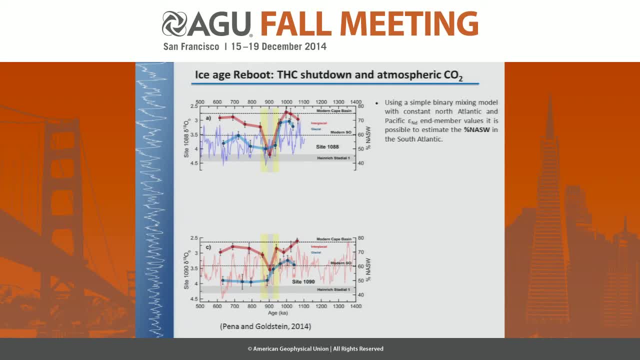 We can use a binary mixing model, assuming constant N-member values in the North Atlantic and in the North Pacific, And we can possibly estimate. We can estimate the percentage of North Atlantic source waters that get into the South Atlantic And, to give you a reference, this is the modern Cape Basin mixing proportions: around 75 percent. 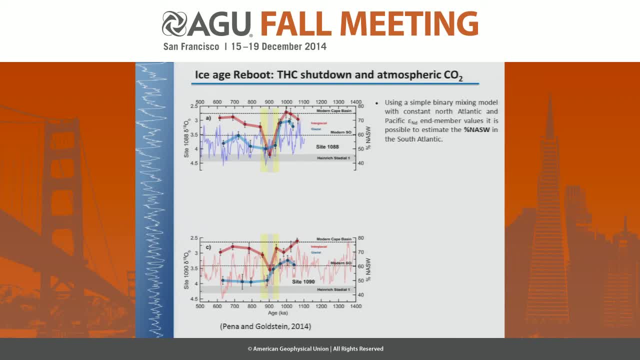 At the modern Southern Ocean. we have around 60 percent here And this would be the values that you would expect during Heinrich's Stadial 1.. So just to put it into context, when we look again at the MIS-23 here and we compare the 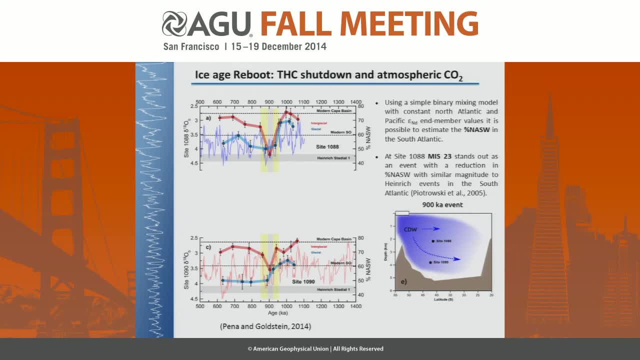 relative proportion of efflorescence. So this is the average number of North Atlantic source water that reaches this site at that time. It's comparable to the values that you would expect in the South Atlantic during Heinrich's Stadial 1, based on previously published epsilon edemium data in the vicinity. 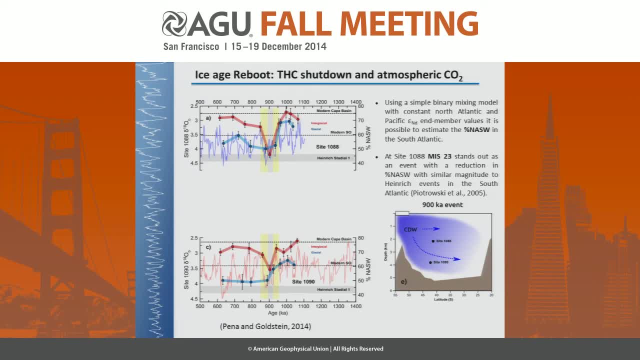 And this is just, you know, amazing that you can have such a reduction in the presence of North Atlantic source waters during this time interval. that would correspond to a scenario that we would like to picture in something like that And, what is even more striking, 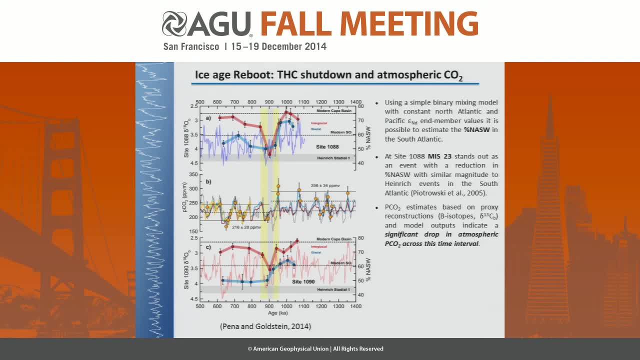 Is that when it's actually during this time interval here that proxy records of atmospheric CO2 and model reconstructions show the largest shift on the largest drop in atmospheric CO2 across that interval. So I mean, to me that's definitely not a coincidence. 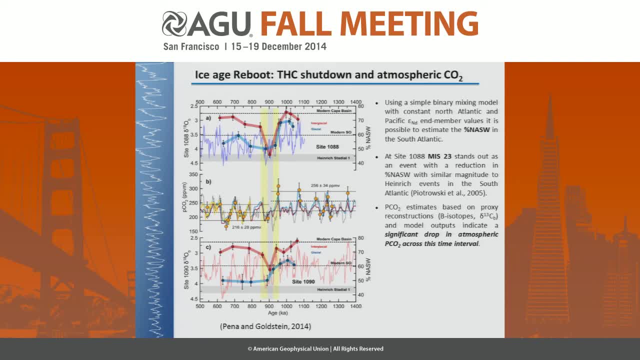 There must be some process going on here that really helps to, that really links together this reduction. I mean it's not a coincidence, but it's not a coincidence, but it's not a coincidence that there is a reduction in thermohaline circulation and the drop of atmospheric CO2.. 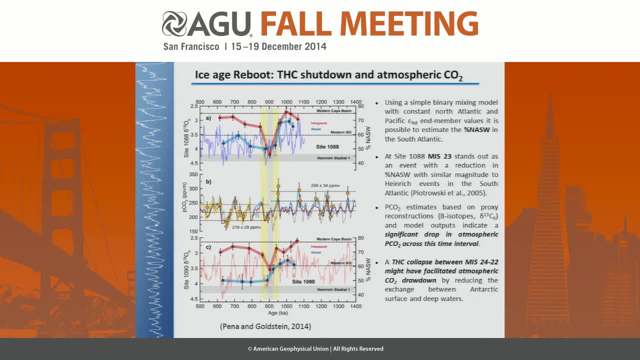 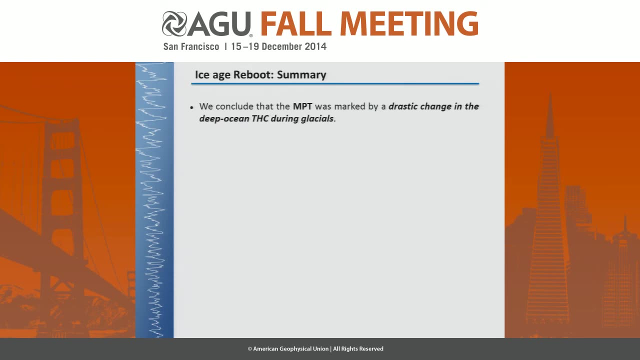 And we could even argue that this THC slowdown or collapse between MIS 24 to 22 might have facilitated the atmospheric CO2 drawdown by reducing the exchange between the Antarctic surface and the deep waters. So, in summary, we conclude that the mid-Pleistocene transition was marked by a drastic change. 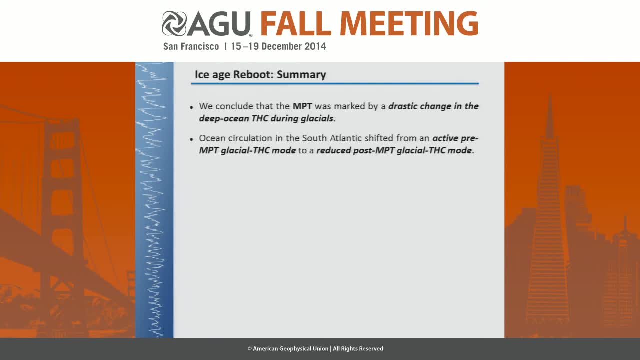 in the deep ocean thermohaline circulation. during glacials, The ocean circulation in the South Atlantic shifted from an active pre-NPT glacial mode into a reduced post-NPT glacial THC mode. In contrast, the vigor of the THC pre- and post-NPT has remained similar during interglacials. 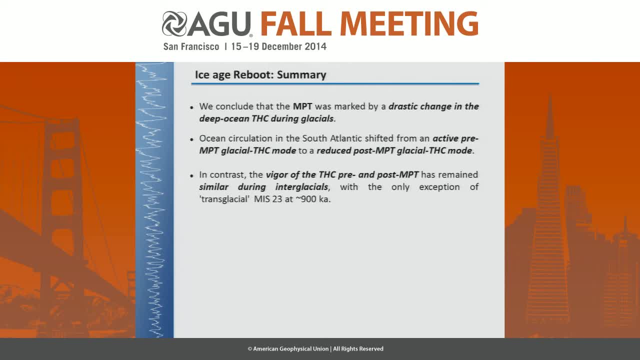 with the only exception of the transglacial MIS 23 at around 900 kilo years. The weak glacial thermohaline circulation might have facilitated the atmospheric CO2 drawdown by reducing exchange between the surface and deep waters, and this affects. 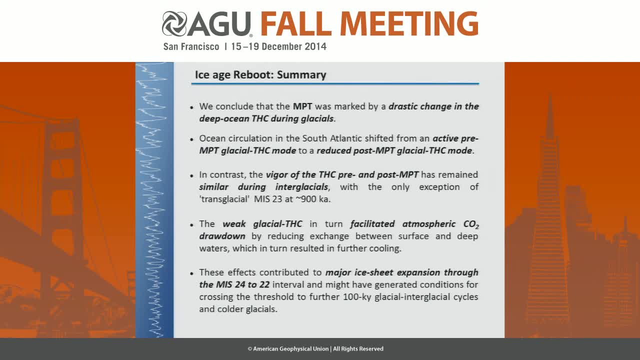 altogether. However, it might have contributed to a minor ice sheet expansion through this time interval. that might just generate the conditions to cross the threshold to further the 100-kilo year glacial and interglacial cycles. And that's it, Thank you. 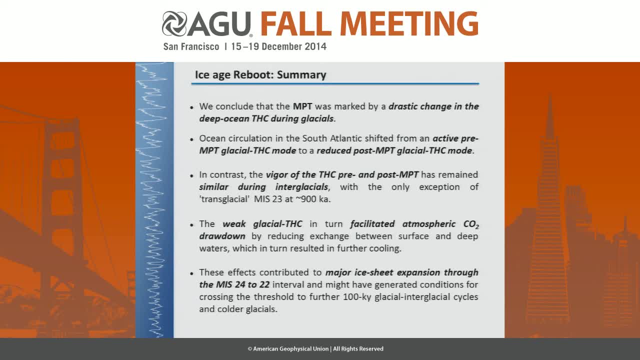 Male Speaker: 1. Thank you very much, Leo. We have time for questions. I've got a question. Male Speaker- 2. Male Speaker. 3. Male Speaker. 4. Male Speaker. 5. Male Speaker. 6. Male Speaker 7.. 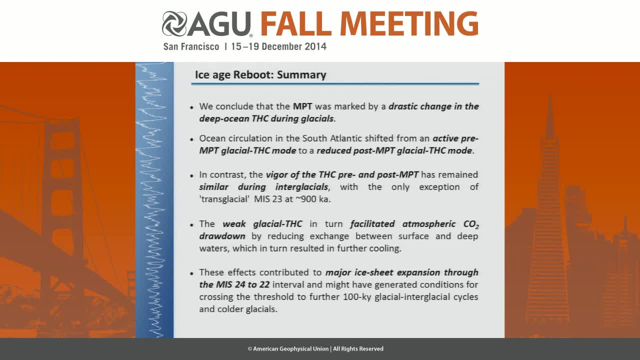 Male Speaker, 8. Male Speaker, 9. Female Speaker, 10. Female Speaker, 11. Female Speaker, 12. Female Speaker, 13. Female Speaker, 14. Female Speaker, 15. Female Speaker, 16. Female Speaker, 17. Female Speaker 18.. 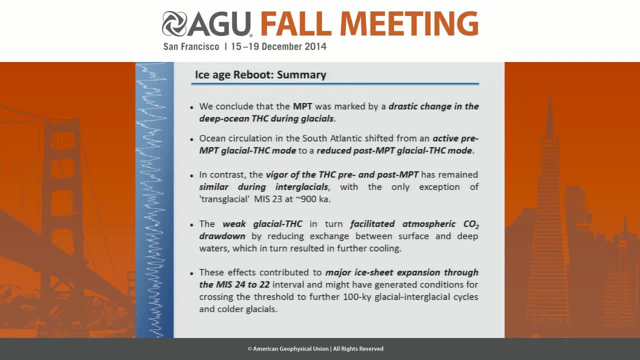 Female Speaker, 19. Female Speaker, 20. Female Speaker, 21. Female Speaker, 22. Female Speaker, 23. Female Speaker, 24. Female Speaker, 25. Female Speaker, 26. Female Speaker, 27. Female Speaker, 28. Female Speaker, 29.. 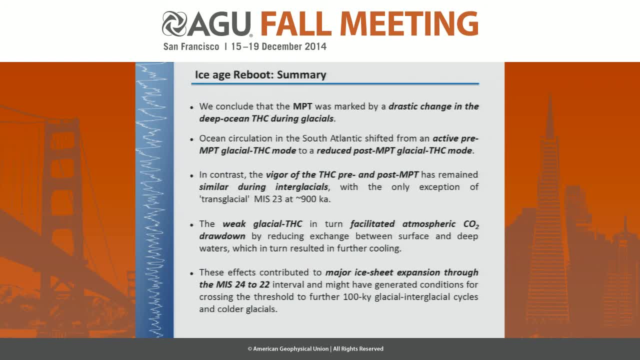 Female Speaker 30.. Female Speaker 31. Female Speaker 32. Female Speaker 33. Female Speaker 34.. Female Speaker 35.. Female Speaker 36. Female Speaker 37.. Female Speaker: 38.. This is actually a work in progress and we hope to have high-resolution records almost. 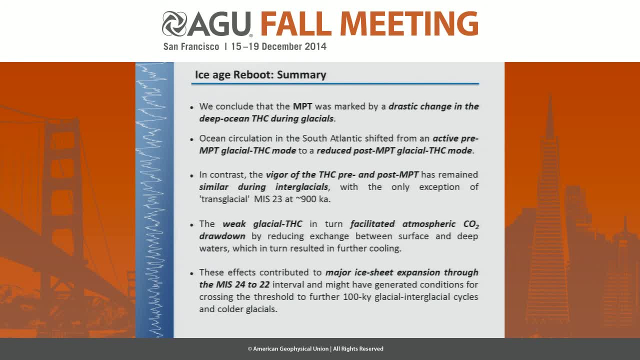 comparable to oxygen isotope records in the near future, And when that happens, I might be able to answer that question. Male Speaker 2. Any more questions? I was tempted to ask a question. I think we have time. You listed some different options for how the mid-placing transition might have been. 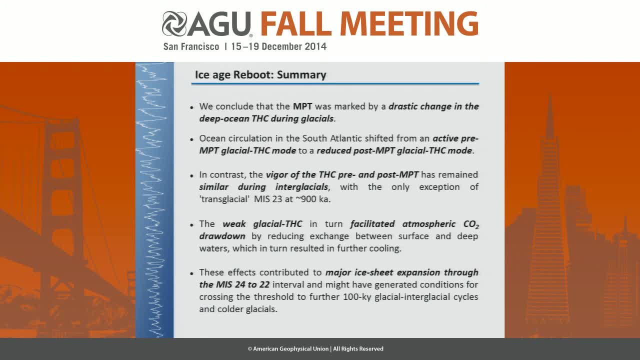 brought about regular hypothesis, that kind of thing, And I was wondering if you could be tempted to kind of comment on how this might connect with those propositions. And you've highlighted the contribution of your changes to an ice sheet expansion. but could it be the other way around? 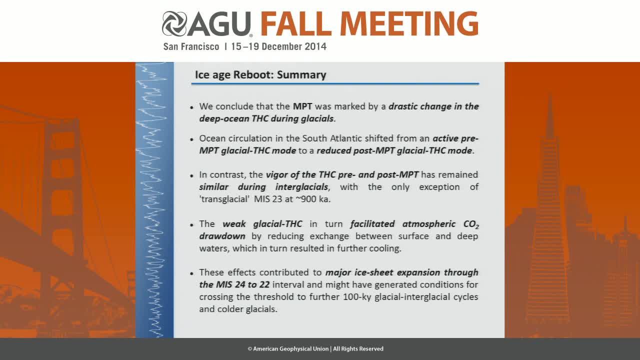 Does it place any constraints on those hypotheses? Male Speaker. 3. Right, I mean, I think everything is linked. It's just, it's like the chicken and the egg. You know, it's really hard when this resolution, in these records, to try to establish lead. 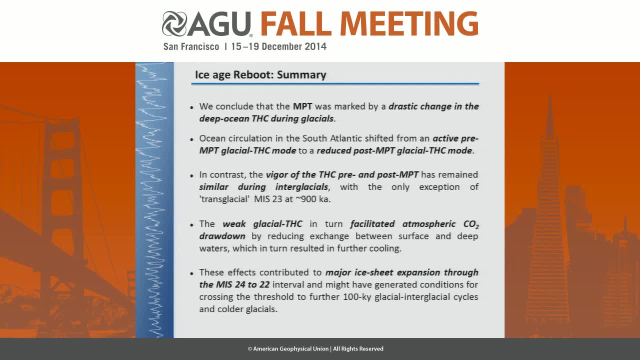 and lags between processes Or what. What is causing what? But there is definitely a link between atmospheric CO2 and deep ocean circulation, And that might have also a feedback effect on the global temperatures, therefore promoting bigger and thicker ice sheets and so on. 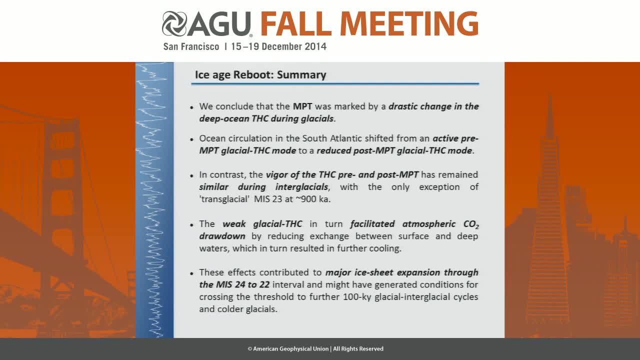 So everything is connected, but you know, we are still not at the point that we can establish this lead-lag relationship. Male Speaker 4..